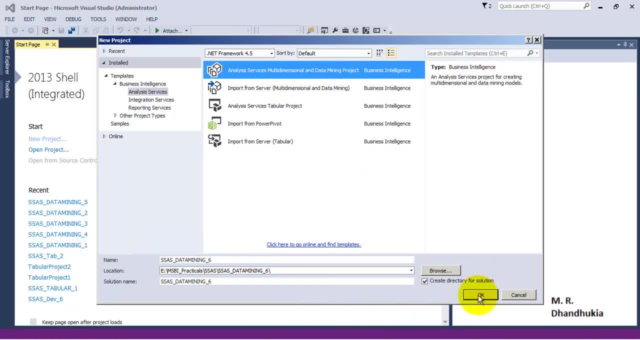 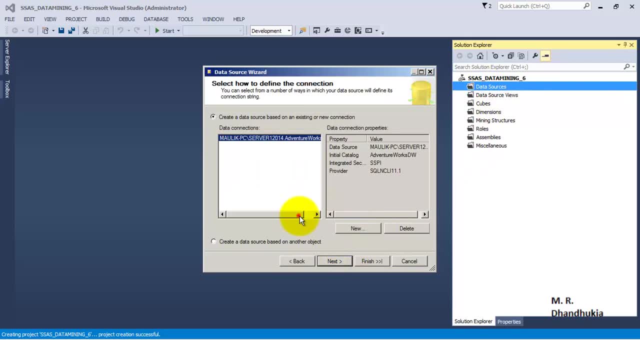 Right, Let us create a new connection. that is data source to Adventure DataWorks DW. So it is pointing to the right database, So let us click next. Let us use service account. Finish. Let us create a new DSV. 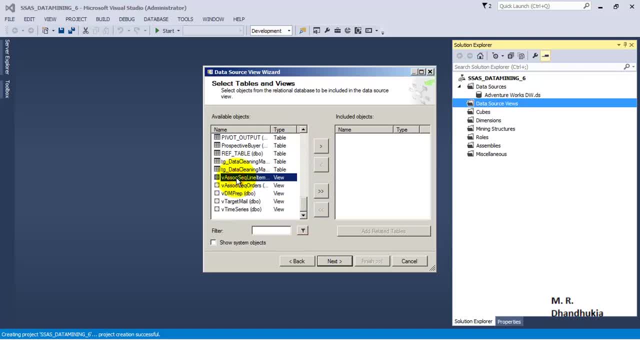 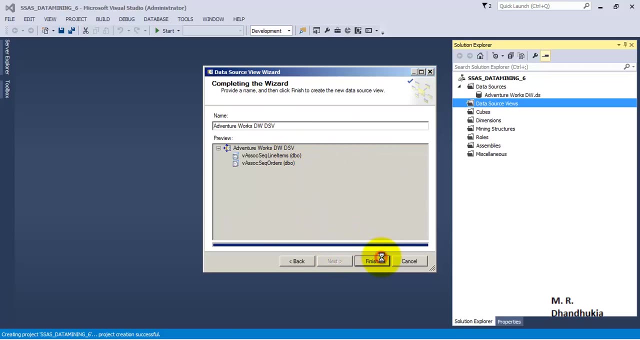 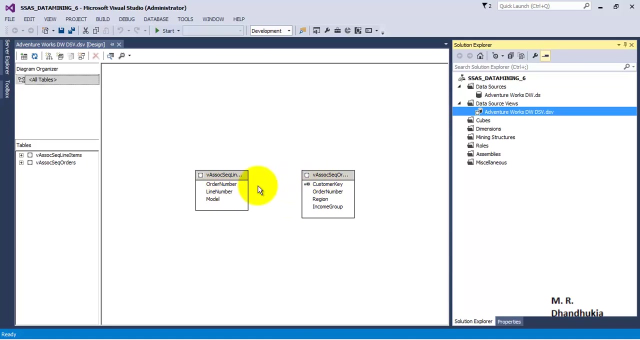 Now let us use the same two views that we have used earlier, Just in our last example, that is, the view related to orders and the line items. Next, Let us call it as DSV Finish Now, as these are views, so there can be foreign key relationship between views. 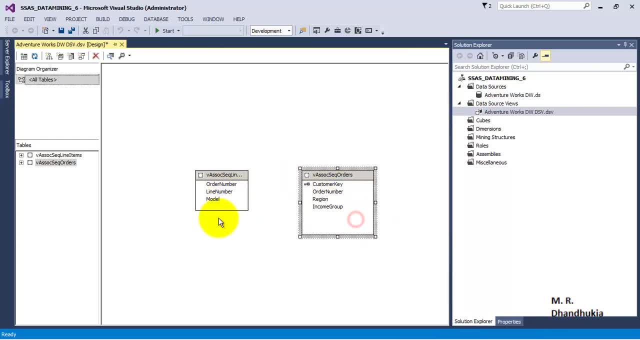 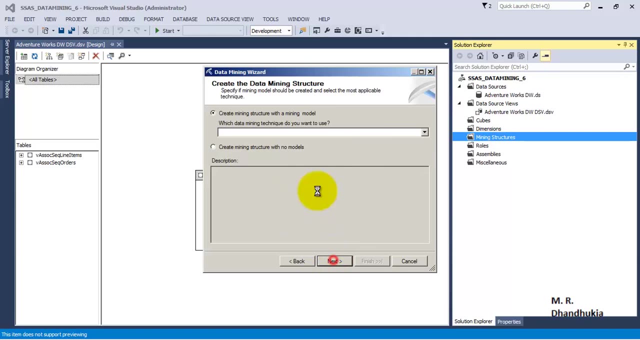 Right. So let us create a logical relationship between these views. This is orders table, This is line items table. So let us create a new view, Let us create the logical relationship. Now let us go and create a new mining structure. 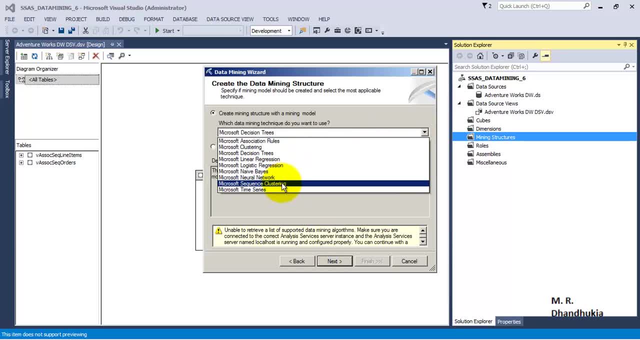 So let us go and select sequence clustering. Now, when is sequence clustering used? Generally, sequence clustering is used to form clusters where the sequencing of events is useful or is important. For example, let us say, if we are analyzing data of sales from a website. 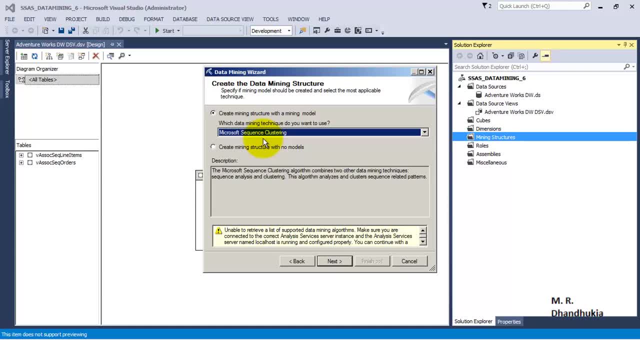 Okay, That is web-based sales. Now, in the website, the sequence of the web pages visited by the customer is important. So the sequence in which the customer bought things over the website, the sequence of pages through which the user travels and kept on buying things, it is important for us. 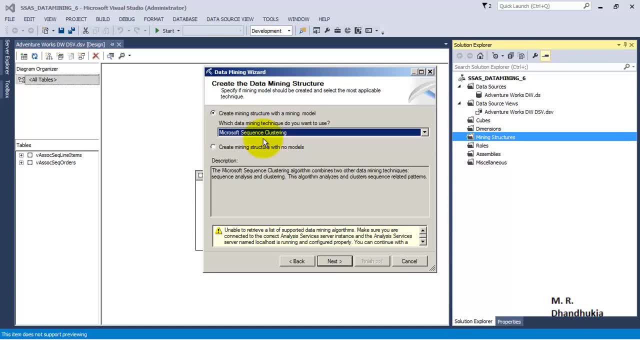 Okay, So that is the way in which we can restructure the website, Okay, Or its flow, content flow. So in such scenarios, generally, the sequence clustering is useful. That is, the scenarios in which we want to, let us say, study the sequence of sales. 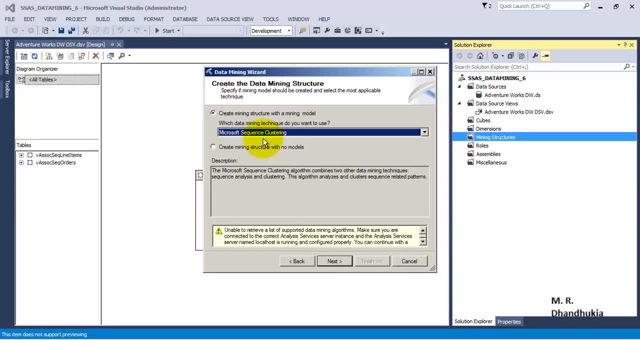 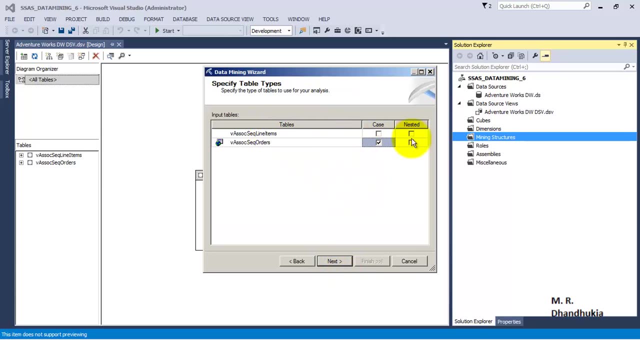 Okay, We are not only interested in the items which have been purchased, but the sequence in which the items have been purchased. Right, If we are interested in that also, then sequence clustering can be used. Let us click next. Next Orders is our main table. 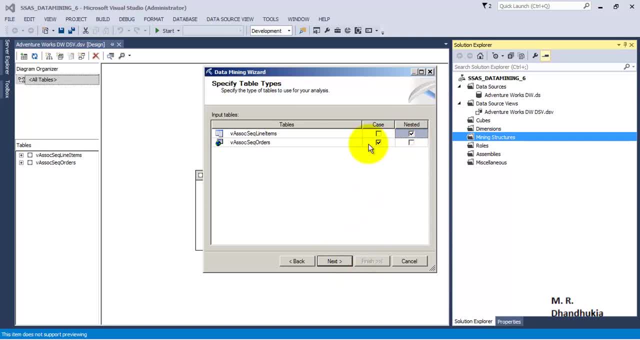 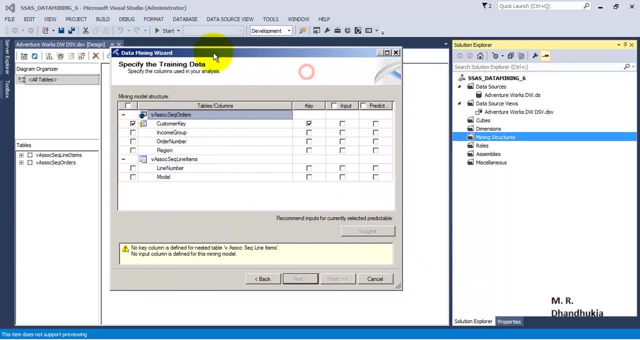 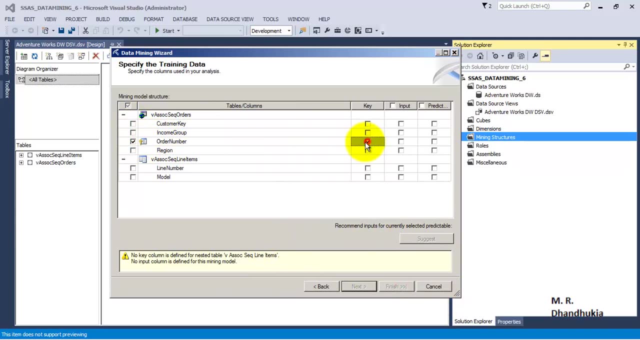 And line items is our supporting table. That is nested table, Right Detailed table. Correct, Now over here. order is the key. Okay, Now over here. in this example, the line number. The line number represents the sequence in which the items have been bought. 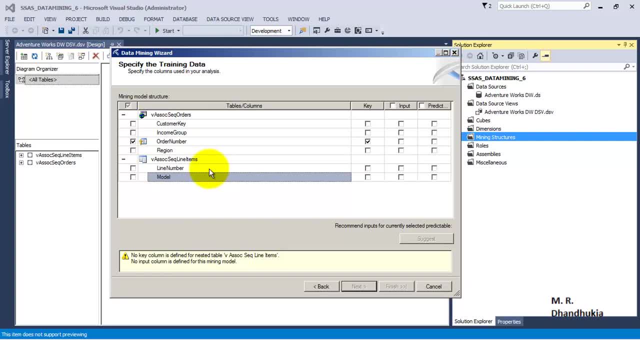 Okay, The model items have been bought in the order of line number, So line number will form part of the key. Okay, So it is also part of the key. Also, what is acting as an input, along with the sequence in which the things have been bought? 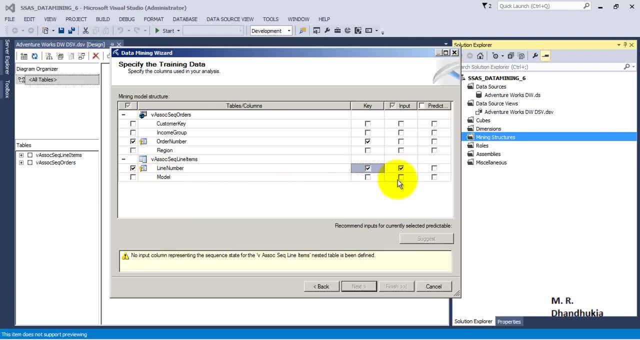 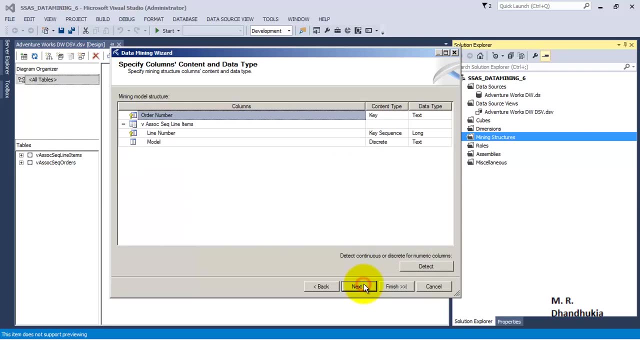 That is line number. Along with that, the actual name of the products that have been bought is also an input Right. So the name of the products is the thing that we want to predict. Okay, So things have been configured in this. 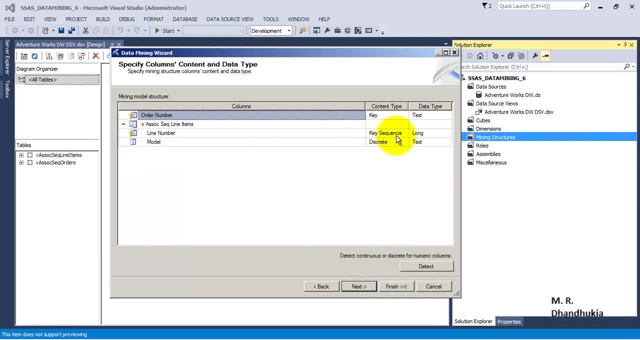 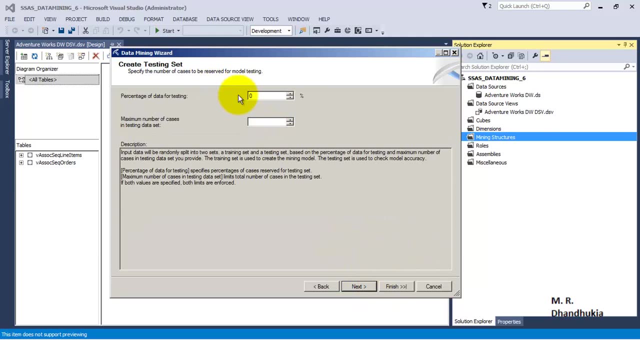 Now, this is correct. Order number is key. Line number is representing the sequence for the key And model is a discrete value which we want to predict. also Right, Let us use all the data. Let us not keep any data for testing purpose. 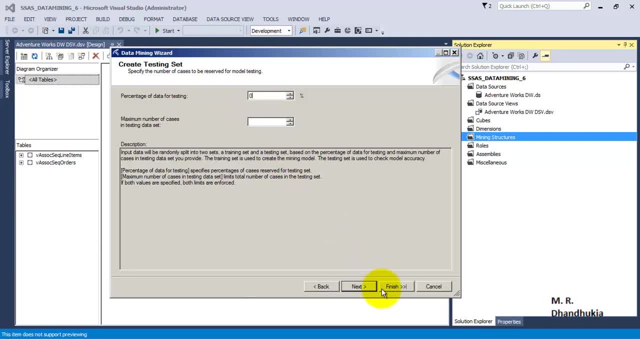 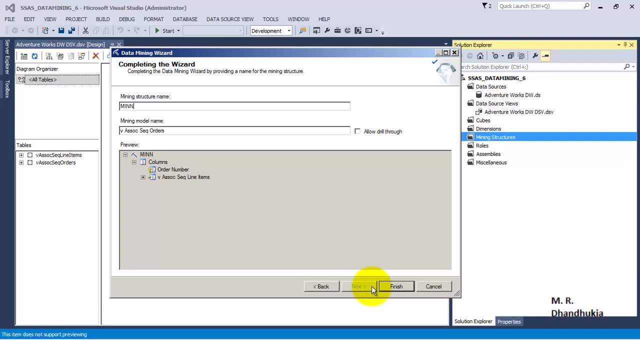 Right, We do not have any test data. We are using the whole data set, Right? Let us call this as mining structure And let us call this as sequence clustering, Right? Okay, So mining model is now prepared, So let us go to database. 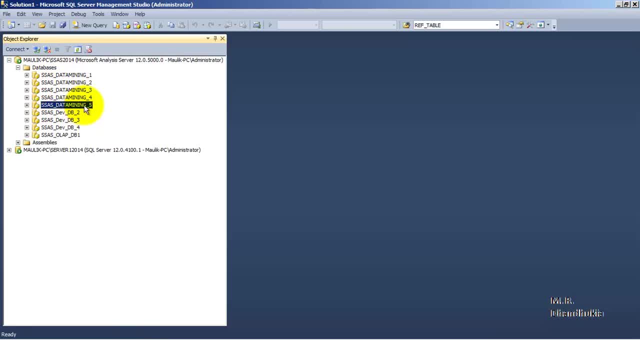 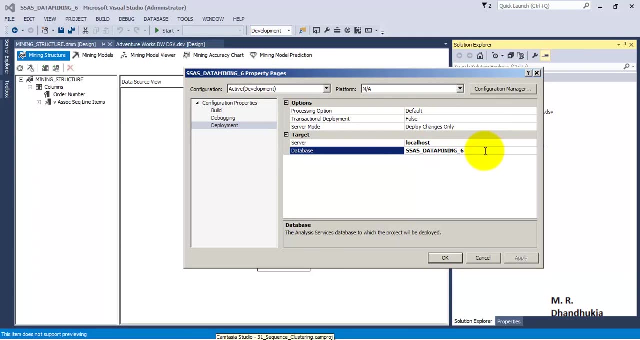 We can see that there is no database with the name SSS data mining 6.. Correct, So let us copy the name. Let us go to deployment properties. We can see that the new database that will be created will be created with the name of 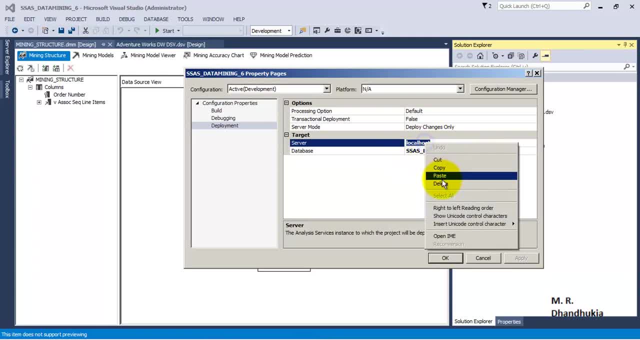 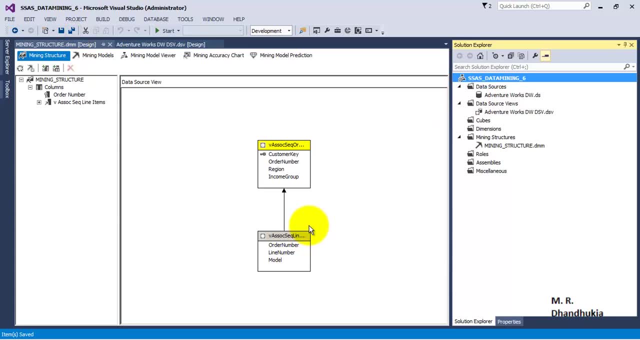 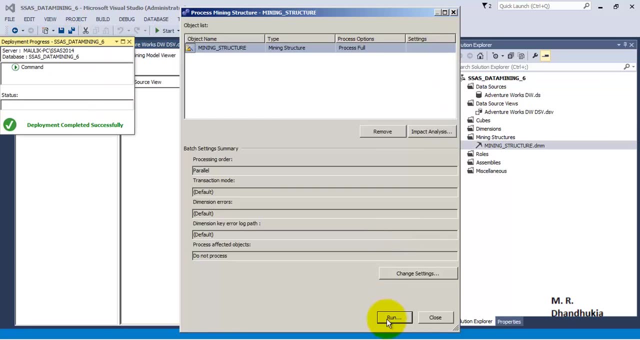 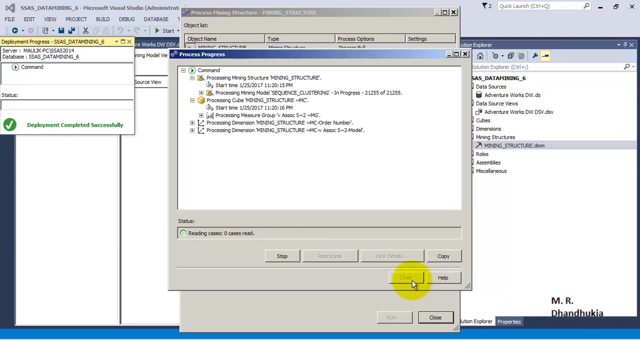 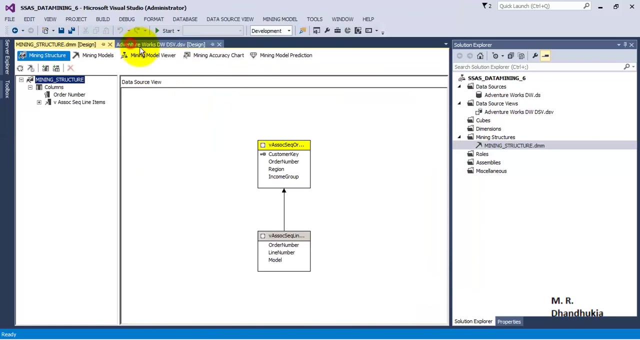 SSS data mining 6.. Right, So let us provide the server name. Right, Okay, Now we can deploy. So deployment and processing has succeeded. So let us close everything, Let us go to database, Let us refresh. 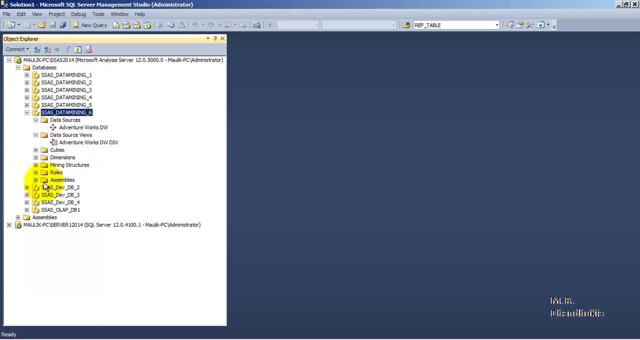 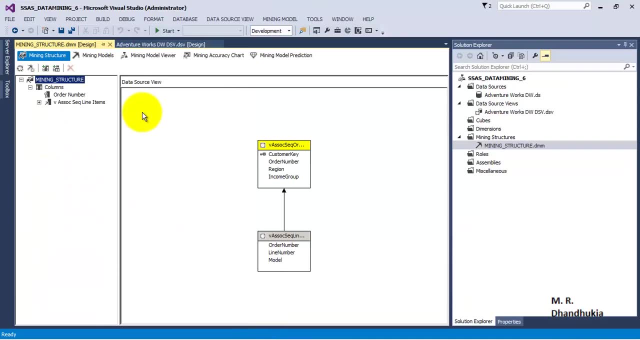 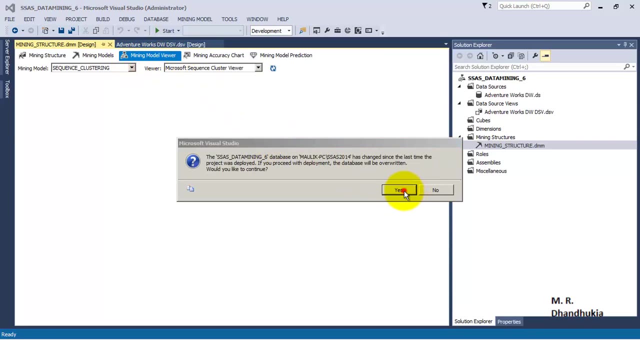 Let us see that things have come to database. Yes, Mining structure also. We can see sequence clustering. Right, So let us go. Now we can go and go through our mining model viewer. Okay, To analyze the data. Okay. 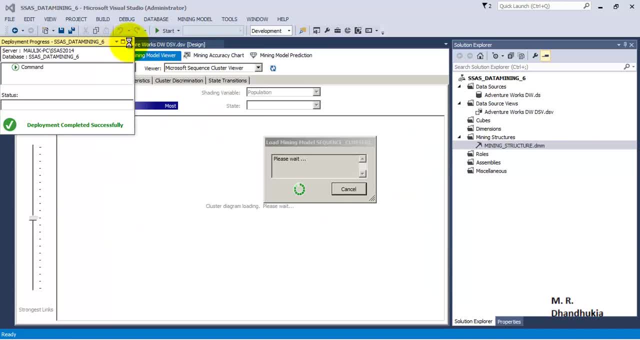 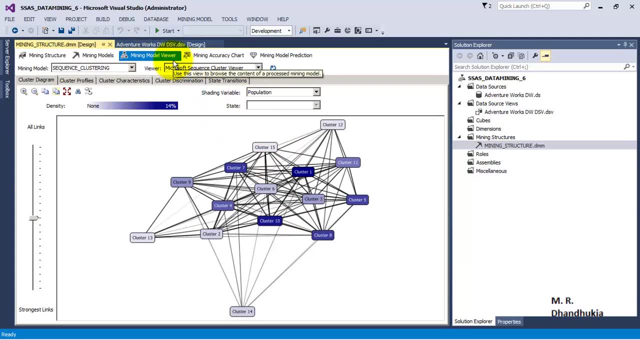 So, as we can see, it is quite similar to the Microsoft clustering algorithm. Okay, So this sequence clustering also forms clusters, But basically it forms clusters based on the sequence of the data, Right, In this case, it is forming sequence of the products which have been purchased. 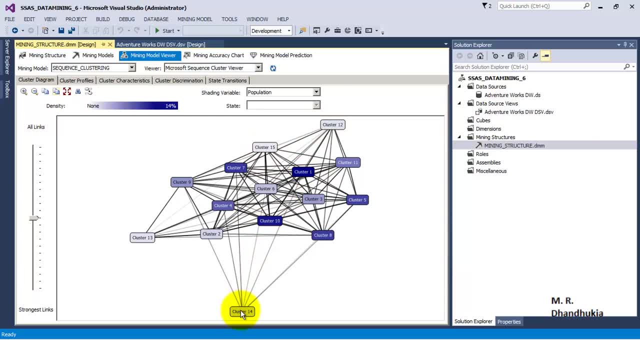 Right, So we can see more than 10 clusters. In fact, 15 clusters have been created. Okay, So this is for the. this shading is for the whole population. If you want, we can have shading for a particular population. 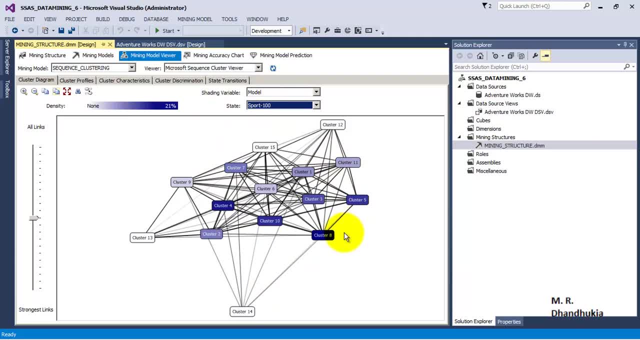 For a particular product also. Let us say 400.. Right. Or let us say mountain tire. Right, So it is only present ML. mountain tire is only present in 13 and 2.. Right Cluster, number 13 and 2.. 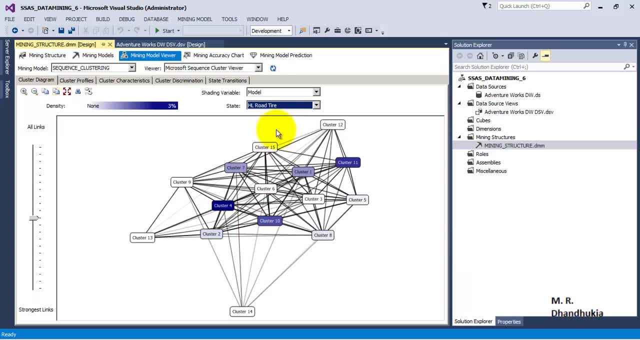 Right, So in this way we can see data product wise also, Right, So LL road tire is present mostly in cluster number 3.. Okay, So in this way also we can analyze the data among the clusters which has been distributed. 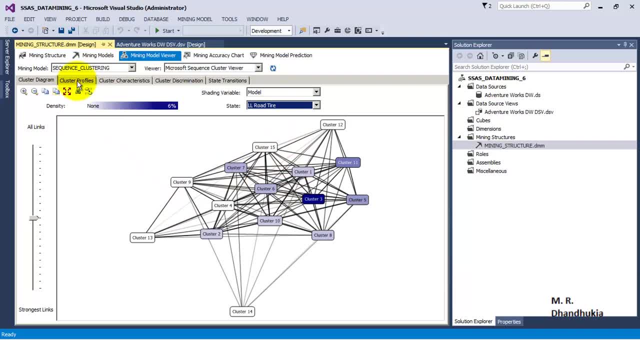 in the cluster. Okay, So now, if you want to study profile of a particular cluster- let us say we want to study profile of cluster number 3, then how can we do that? We go to cluster profiles, We go over here. 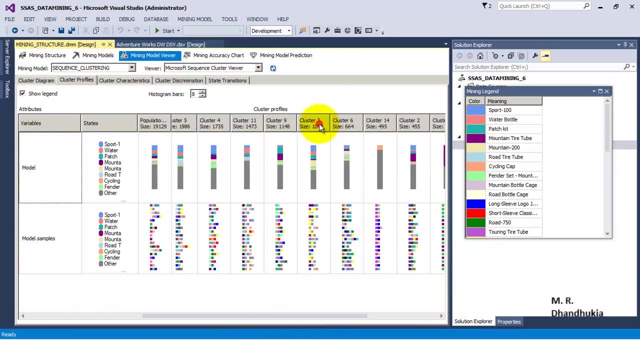 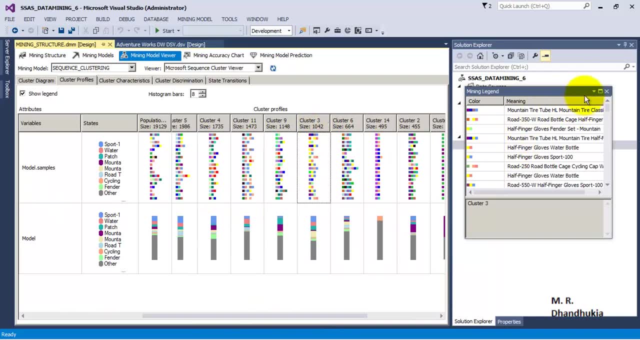 Right, Every column is representing a cluster. We can go over here. This is cluster 3.. And then in cluster 3, we can analyze the data further. Let us go to cluster characteristics. So this is for the whole population. 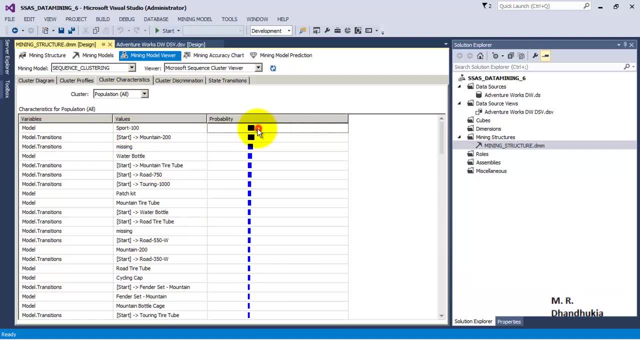 So it shows that models 400 is the one having maximum sales. Right, It is having maximum probability. So if you want to go to cluster 3, then mountain 200 is the starting point. Right. LL road tire is also present. 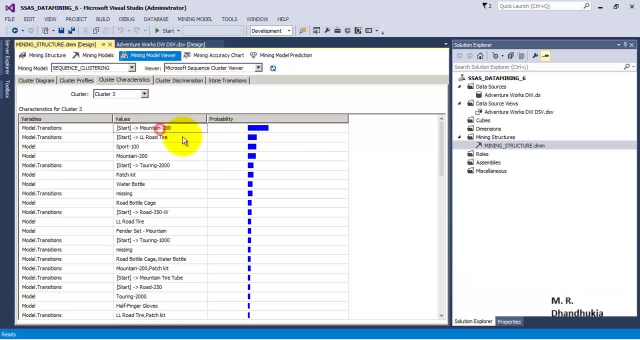 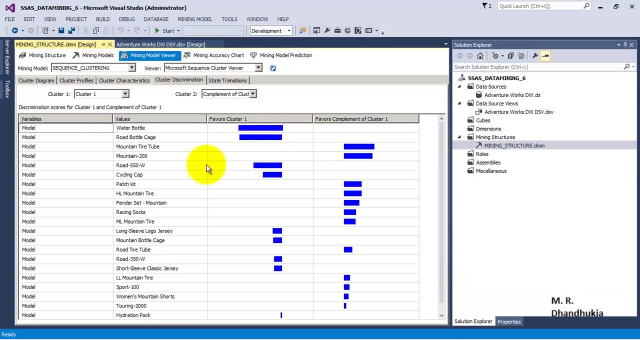 Right. So in this way we can analyze the following: We can analyze the further sequence of transactions in the cluster also Right Cluster discrimination is similar to the diagram or the chart that we had seen as part of clustering Right Over. here we can compare which all attributes are favoring which cluster. 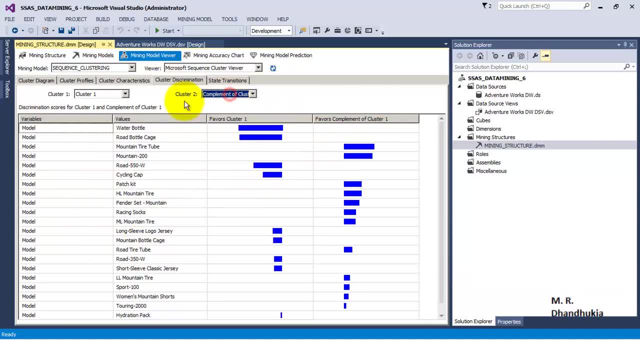 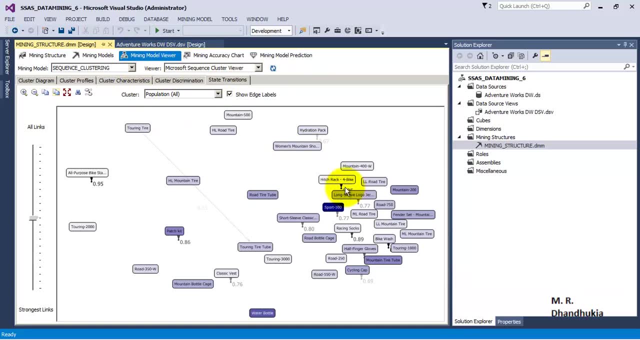 Okay, Or the complement of the cluster. Okay, Right, And this is very important And this is new for the cluster: sequencing Right For sequence clustering. So over here if we let us analyze cluster number 3.. Okay, 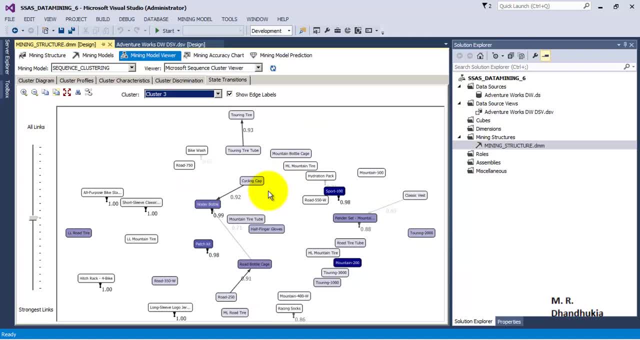 So we can understand that, generally, after cycling cab, there is 92% probability of person buying water bottle. Okay. After buying road bottle cage, there is 99% probability that the person buys water bottle. Okay. After LL road tire right: generally there is 62% probability that person buys patch. 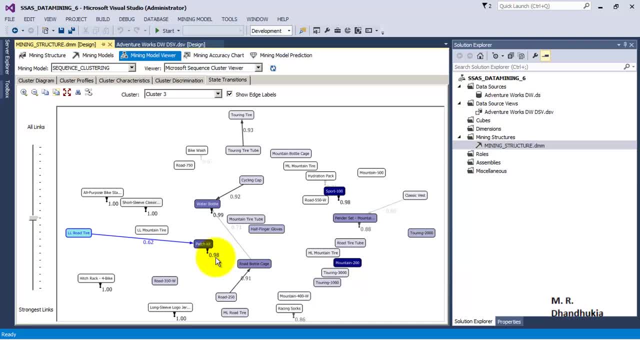 kit And after patch kit, there is 98% probability that the customer doesn't buy anything further. Okay, So this symbol is for AND. Okay, So there is 98% probability that customer doesn't buy anything. So in this way, we can analyze the exact sequence in which customer is buying different. 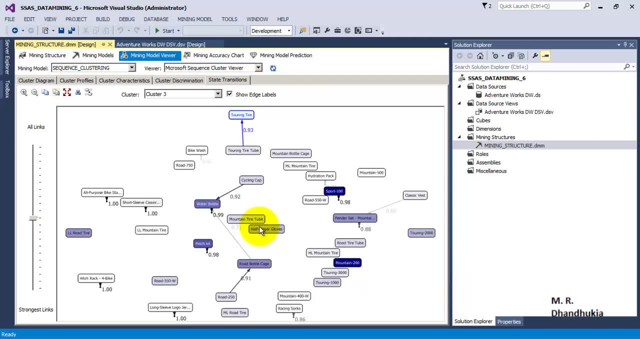 products using the help of state transitions diagram. So this is very helpful and very important for as far as sequence clustering is concerned. So I hope, friends, this video tutorial is useful to you. Thank you.